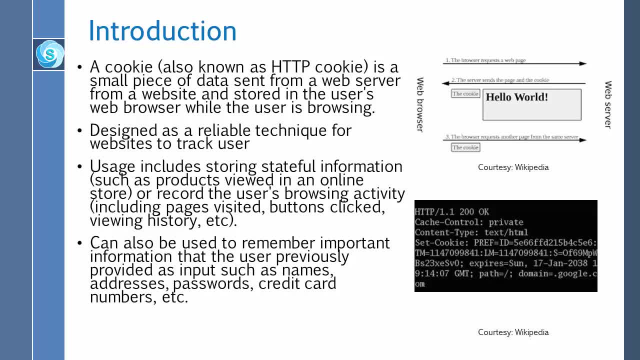 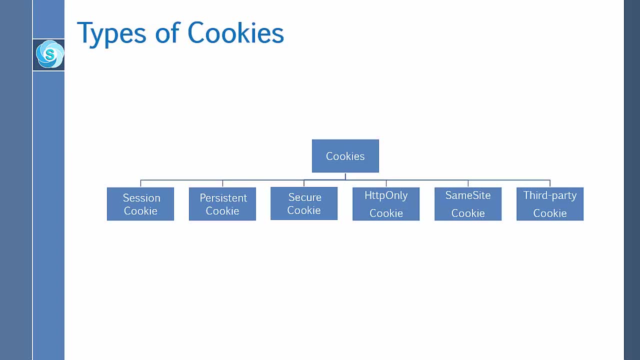 be used to remember important information that the user previously provided as input, such as names, addresses, passwords, credit card numbers, etc. Now I will discuss different types of commonly used cookies. There are mainly Session Cookie, Persistent Cookie, Secure cookie, HTTP only cookie- same. 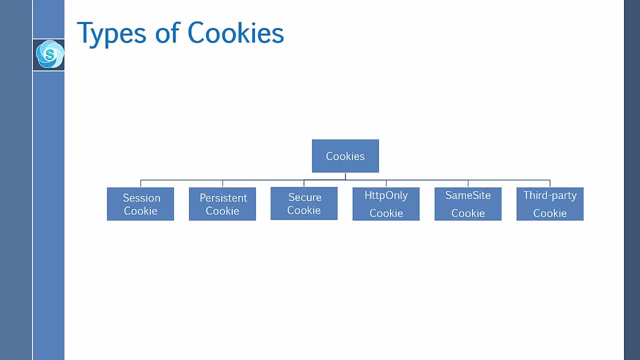 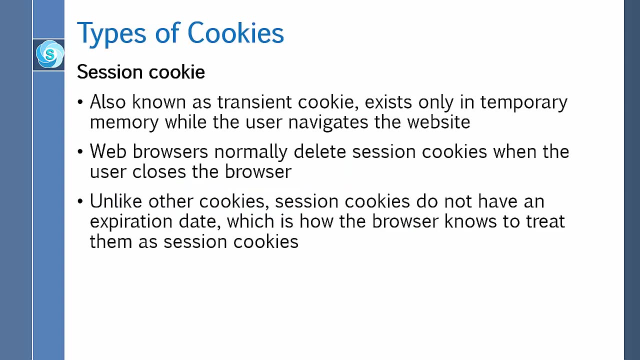 site cookie, third party cookie. There are other types of cookies also, but I will focus only on these cookies as they are widely used in practice. Now let me begin with Session Cookie. It is also known as transient cookie. It exists only in temporary memory, while the 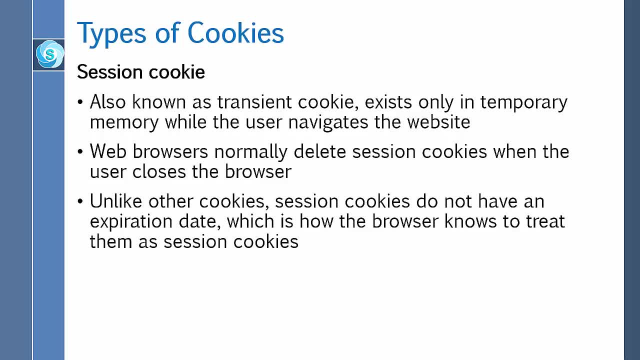 user navigates the website, and that is the main function of the Session Cookie. Now let website Web browsers normally delete session cookies when the user closes the browser. Unlike other cookies, session cookies do not have an expiration date, which is how the browser knows to treat them as session cookies. Now let me talk. 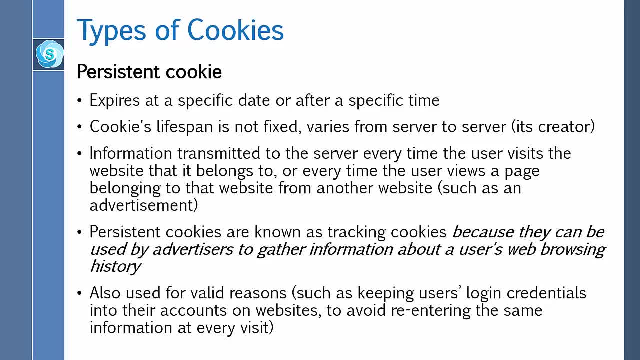 about persistent cookie. It expires at a specific date or after a specific time. Cookies lifespan is not fixed. It varies from server to server. basically, its creator Information is transmitted to the server every time the user visits the website what it belongs to, or every time the user views a page belonging to. 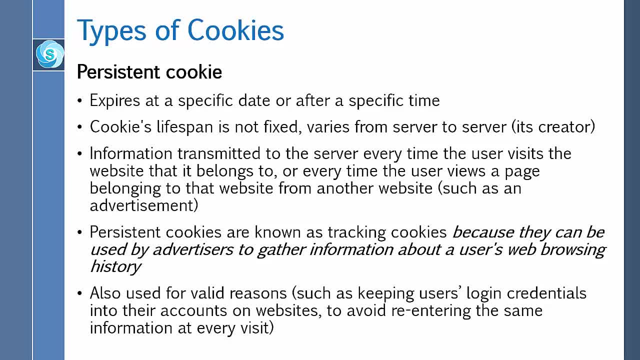 that website from another website, such as an advertisement. Persistent cookies are also known as tracking cookies because they can be used by advertisers to gather information about a user's web browsing history. They are also used for valid reasons, such as keeping users login credentials into their accounts on websites to avoid 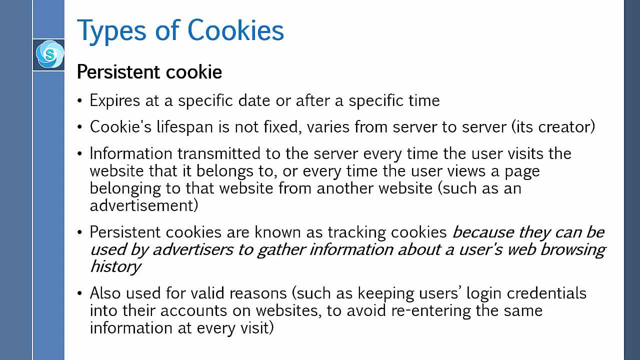 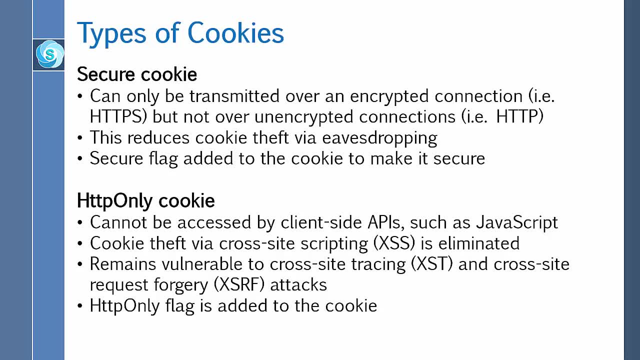 re-entering the same information at every visit. Now let me talk about secure cookie. A secure cookie can only be transmitted over an encrypted connection, that is, HTTPS, but not over unencrypted connections like HTTP. this reduces cookie theft via eavesdropping. a Secure flag is 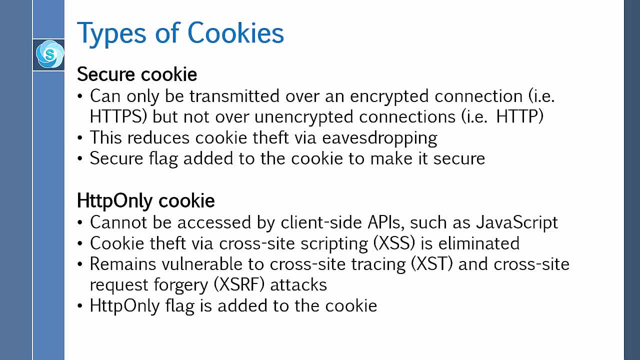 added to the cookie to make it secure. it cannot be accessed by clientsite API such as Javascript. Cookie theft via cross-site scripting is eliminated. It is a type of computer security vulnerability. It is not possible to access it by cloud. It is not possible. 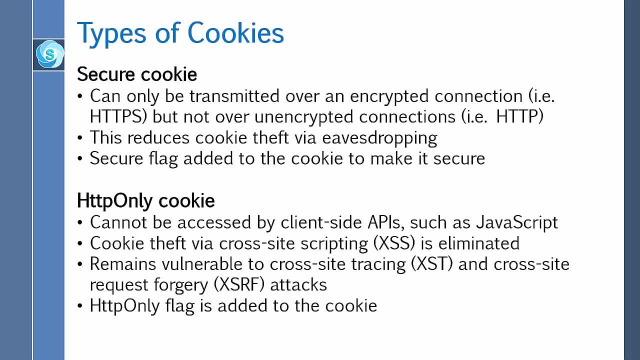 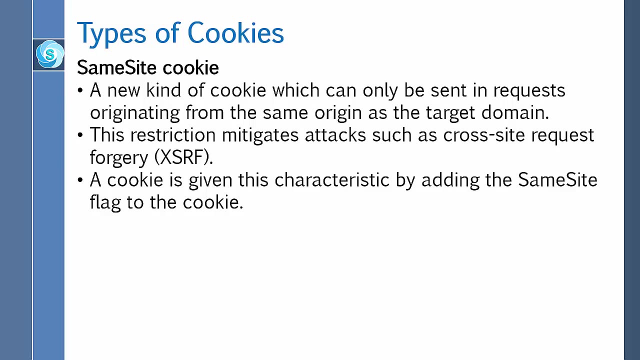 typically found in web applications. Cross-site scripting enables attackers to inject client-side scripts into web pages viewed by other users. However, it remains vulnerable to cross-site tracing and cross-site request forgery attacks. A HTTP-only flag is added to the cookie. Now let me talk about same-site cookies. 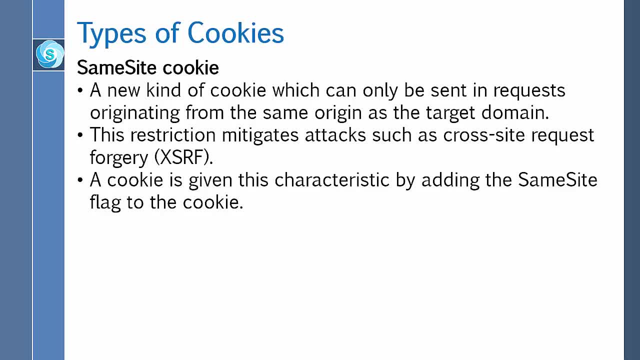 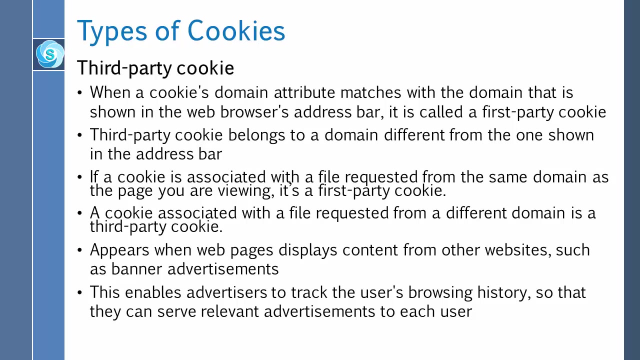 A new kind of cookie, called same-site cookie, can only be sent in request originating from the same origin as the target domain. The restriction mitigates attacks such as cross-site request forgery. A cookie is given this characteristic by adding the same-site flag to the cookie. There is another kind of cookie which is also very popular, called third-party. 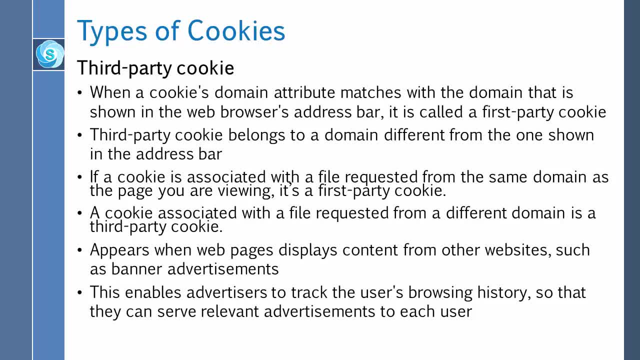 cookie. When a cookie's domain attribute matches with the domain that is shown in web browser's address bar, it's called a first-party cookie. Third-party cookie belongs to a domain different from the one shown in the address bar. If a cookie 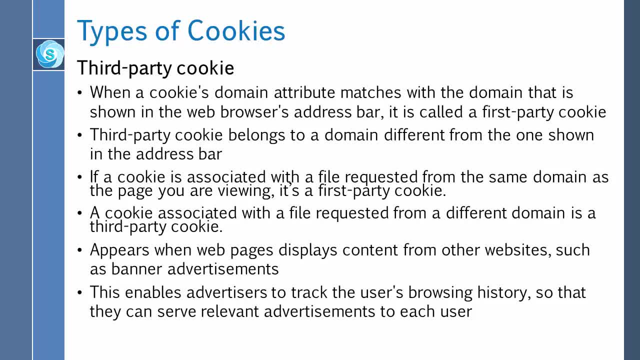 is associated with a file requested from the same domain as the page you are viewing. it is called first-party cookie. A cookie associated with a file requested from a different domain is a third-party cookie. It appears when web pages displays content from other websites, such as banner advertisements. It enables advertisers to 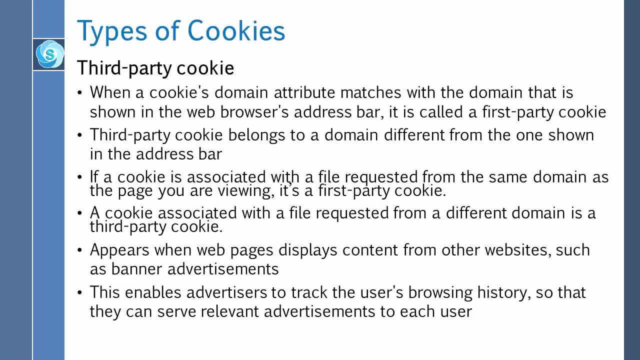 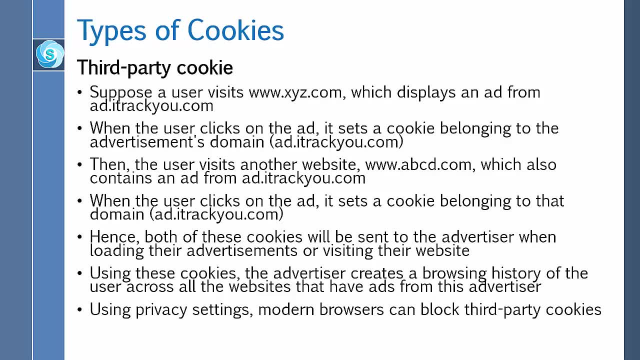 track the user's browsing history so that they can serve relevant advertisements to each user. Now let me explain what a third-party cookie is by giving you an example. Suppose a user visits wwwxyzcom, which displays an ad for a third-party cookie. When the user clicks on the ad, it sets a cookie belonging to the advertisement's domain. 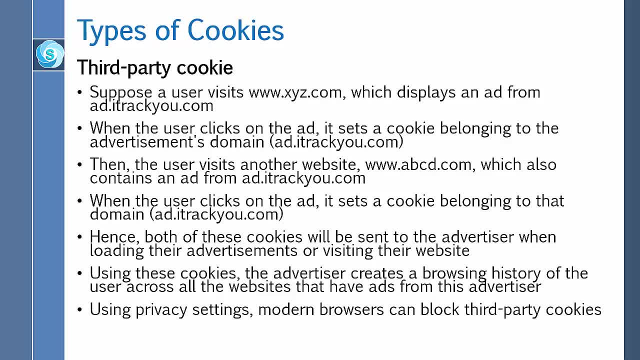 Then the user goes to wwwabcdcom, which also contains an ad from aditrackucom. When the user clicks on the ad, it sets a cookie belonging to the domain aditracucom. Hence, both of these cookies will be sent to the advertiser. 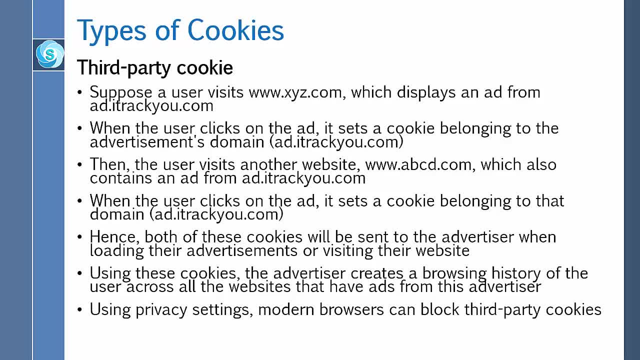 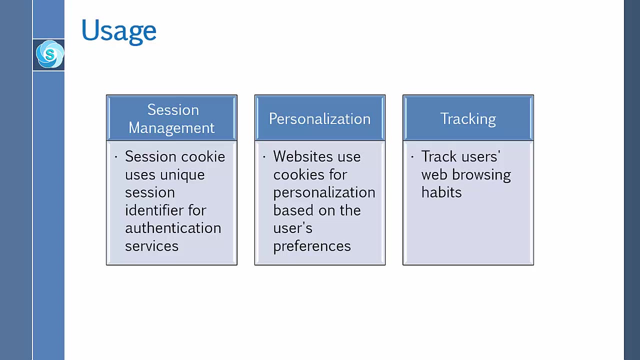 when loading their advertisements or visiting their website. Using these cookies, the advertiser creates a browsing history of the user across all the websites that have ads from this advertiser. Using privacy settings, modern browsers can block third-party cookies. Now let me discuss some of the usage of cookies. 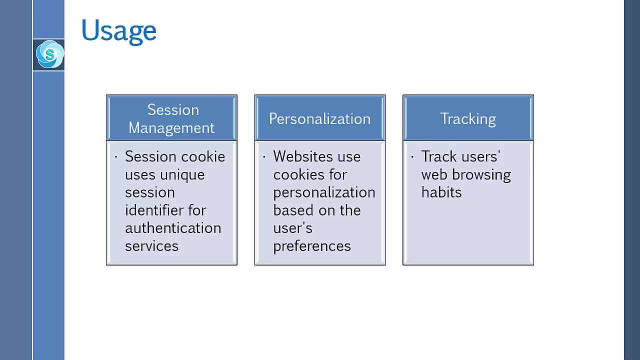 The main usage of cookies are as follows: Session management, personalization and tracking. For session management: Session Cookie uses unique session identifier for authentication services. For personalization, websites use cookies for personalization based on user's preferences. And for tracking: cookies are used to track users'. 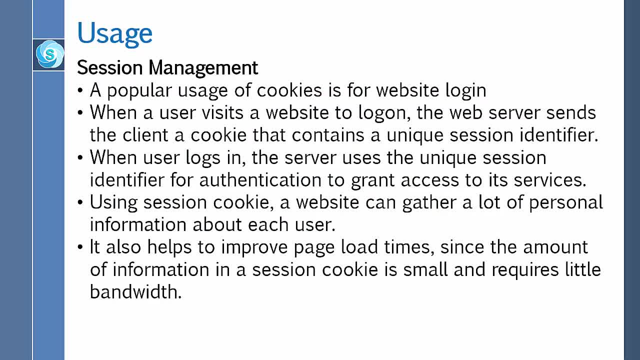 web browsing habits. Now let me talk about session management. A popular usage of cookies is for website login. When a user visits a website to log on, the web server sends the client a cookie that contains a unique session identifier. When a user logs in, 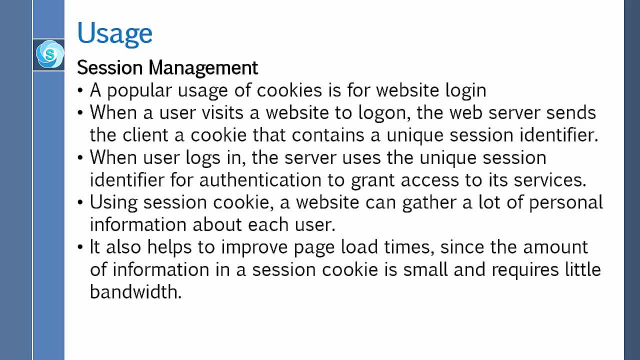 the server uses the unique session identifier for authentication to grant access to its services. Using a Session Cookie, a website can gather a lot of personal information about each user. It also helps to improve page load times, since the amount of information in a Session Cookie is small and requires little bandwidth. 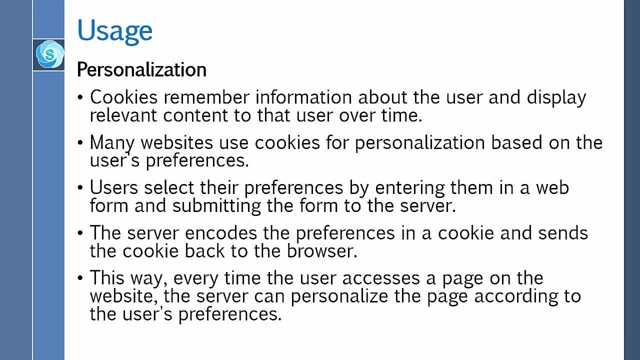 Now let me talk about personalization. Cookies can be processed in several ways. If you are using a web server, you can use cookies to display relevant content to your user over time. Many websites use cookies for personalization based on the user's preferences. Users select their 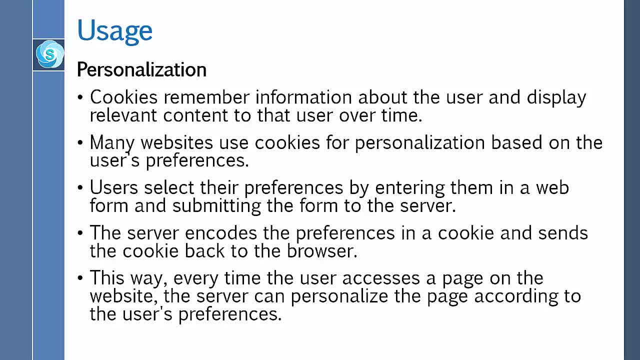 preferences by entering them in a web form and submitting the form to the server. The server encodes the preferences in a cookie and sends the cookie back to the browser. This way, every time the user accesses a page on the website, the, The server can personalize the page according to the user's preferences. 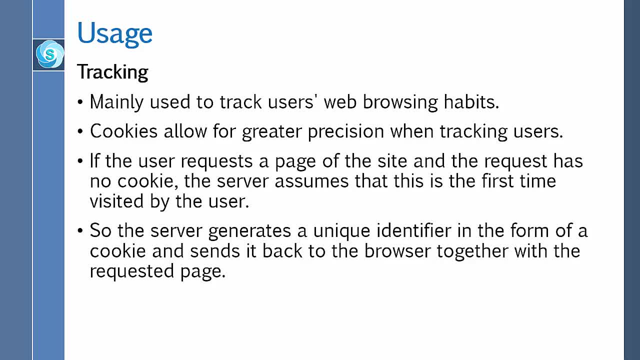 Now let me talk about tracking. It is mainly used to track users' web browsing habits. Cookies allow for greater precision when tracking users. If the user requests a page on the site and the request has no cookie, the server assumes that this is the first time visited by the user. 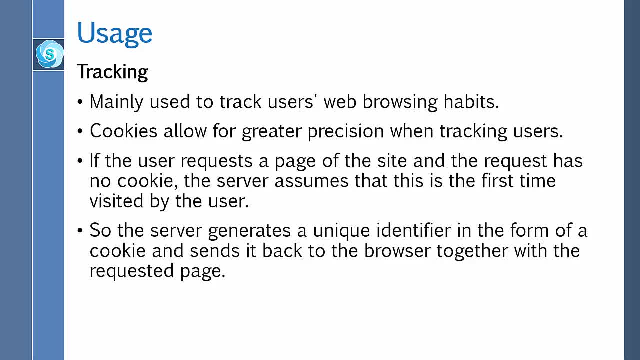 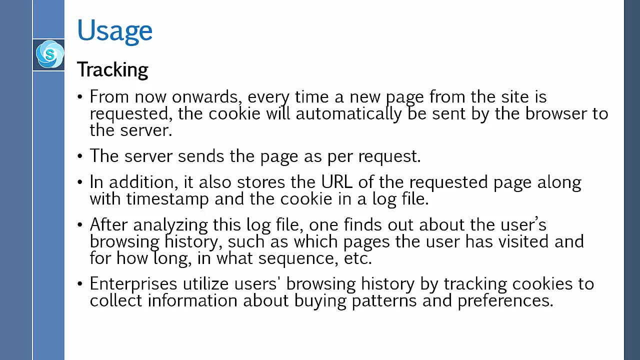 So the server generates a unique identifier in the form of a cookie and sends it back to the browser with the requested page. From now onwards, every time a new page from the site is requested, the cookie will automatically be sent by the browser to the server. 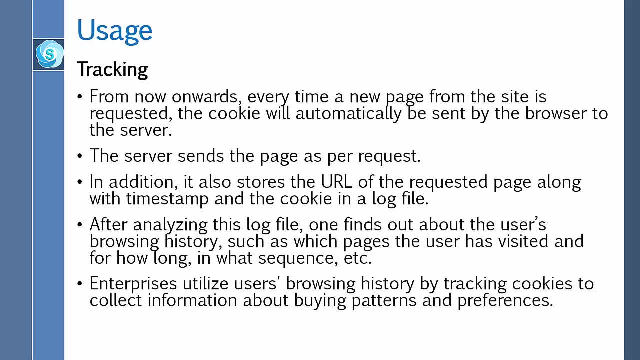 The server sends the page as per request. In addition, it also stores the URL of the requested page, along with timestamp and the cookie, in a log file. After analyzing this log file, one finds out about the user's browsing history, such as pages the user has visited and for how long, in what sequence, etc. 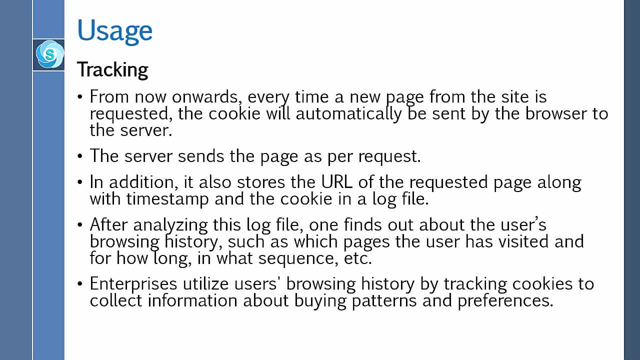 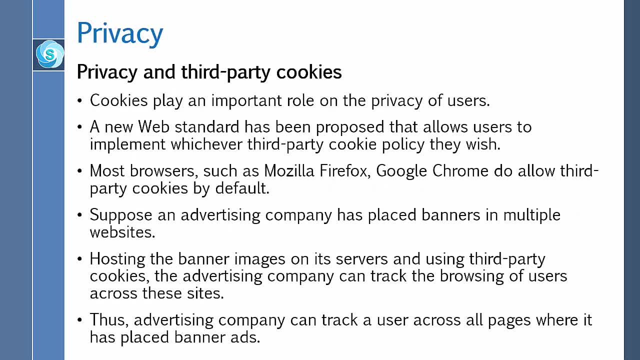 Enterprises utilize users' browsing history by tracking cookies to collect information about buying patterns and preferences. Now let me talk about privacy and third-party cookies. Cookies play an important role on the privacy of users. A new web standard has been proposed that allows users to track cookies. 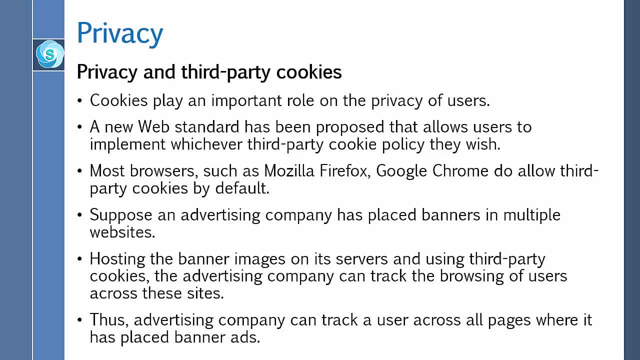 This allows users to implement whichever third-party cookie policy they wish. Most browsers, such as Mozilla Firefox, Google Chrome, do allow third-party cookies by default. Suppose an advertising company has placed banners in multiple websites, Hosting the banner images on its servers and using third-party cookies. 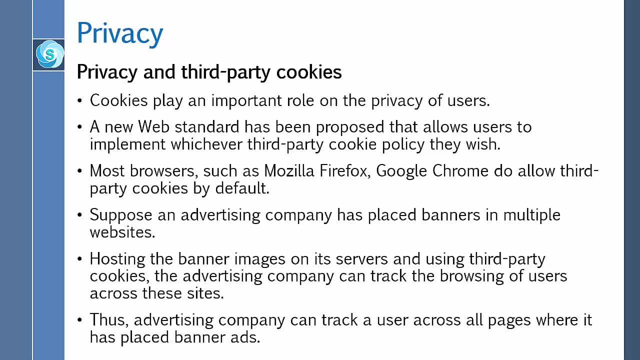 the advertising company can track the browsing of users across these sites. Thus, advertising company can track a user across all pages. This allows users to track a user's browsing history by tracking the number of pages they have visited and the number of banners they have placed in the search results.